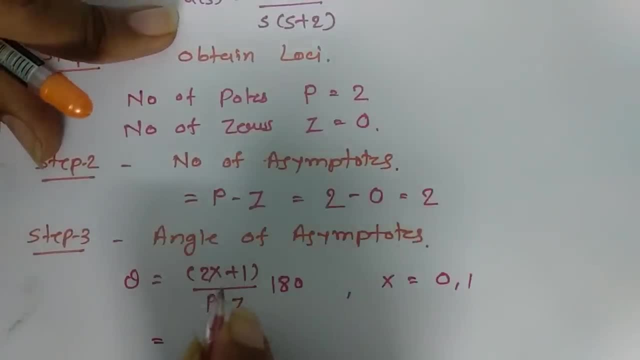 So if I place x is equals to 0 inside, so this will be 1 into 180 divided by 2, so that will be 90, and if I place x is equals to 1.. So this will be 1 into 180 divided by 2, so that will be 90, and if I place x is equals to 1.. 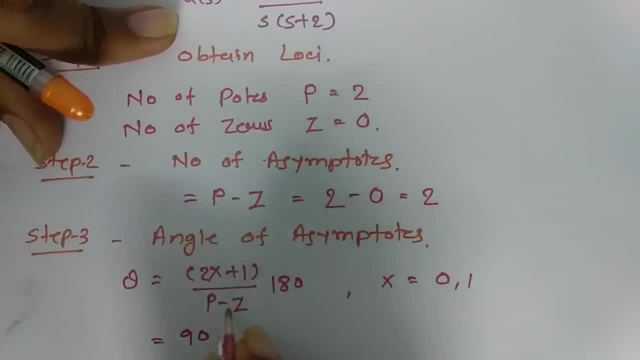 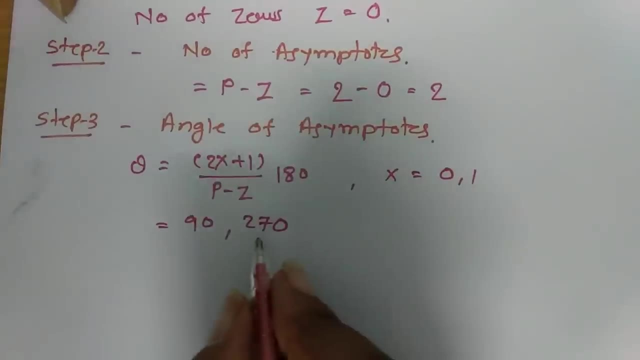 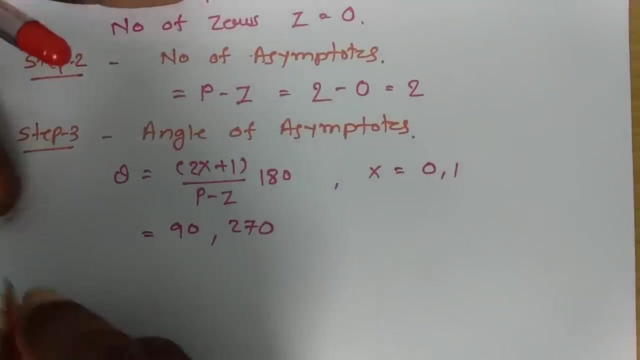 And this will be: 2 plus 1 is equal to 3 into 180 divided by 2, so that will be 270.. So angles of SM totes, that is 90 and 270.. Now next step over here, that is to have a calculation of centroid of SM totes. 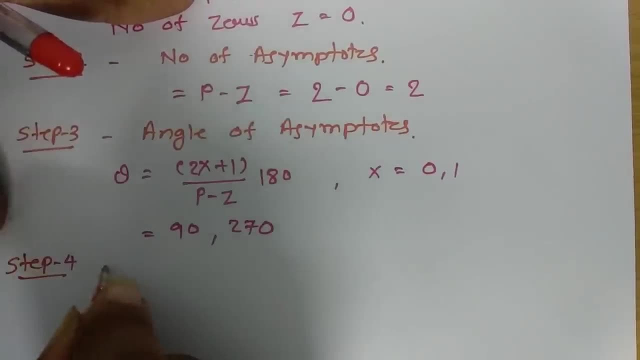 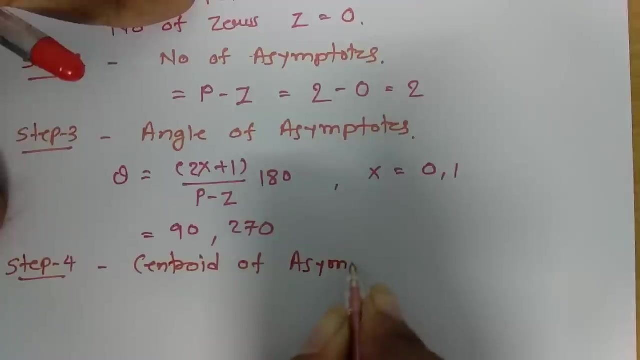 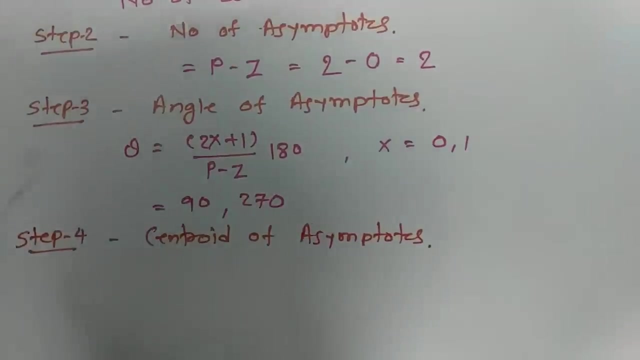 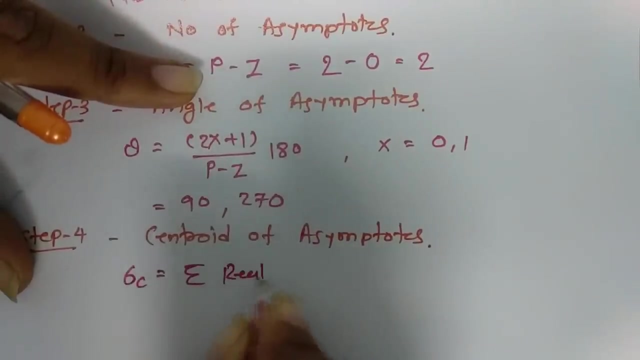 So step number four, that is to have a calculation of centroid of2x asymptotes. So over here for this centroid of asymptotes. centroid of asymptotes is summation of real part of pole minus summation of real part of zeros divided by poles minus 0. So 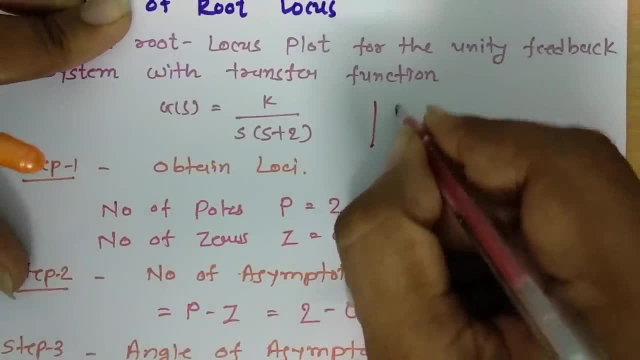 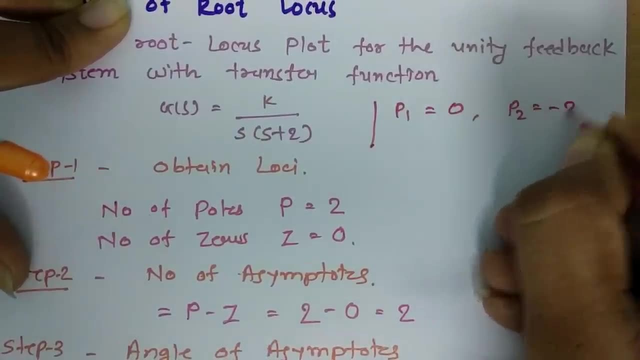 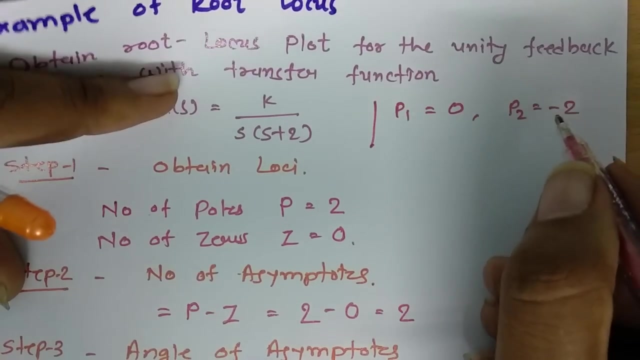 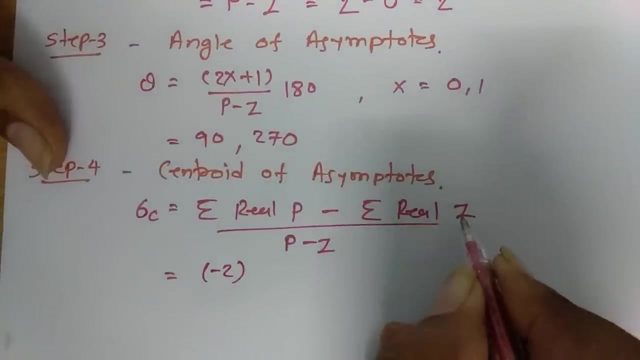 here we have poles: first pole that is there at 0 and second pole that is there at minus 2 and there is no 0. So summation of real parts of poles, that is 0 plus minus 2.. So this is minus 2, and summation of real part of zeros, So that is 0 divided by poles minus. 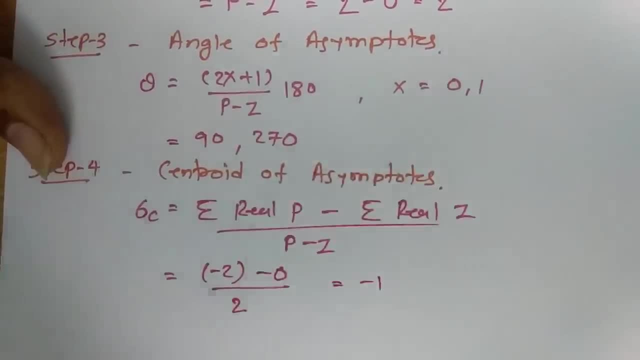 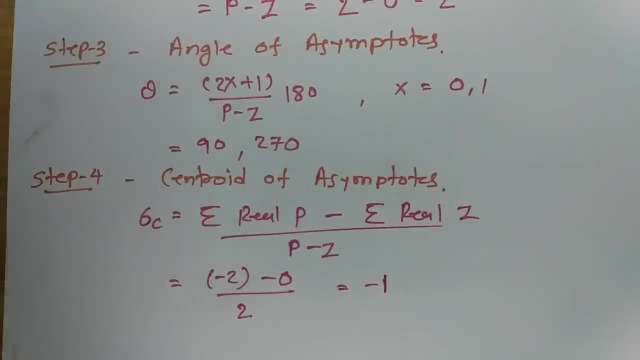 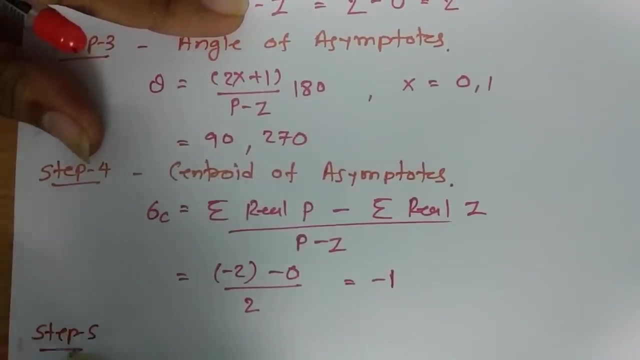 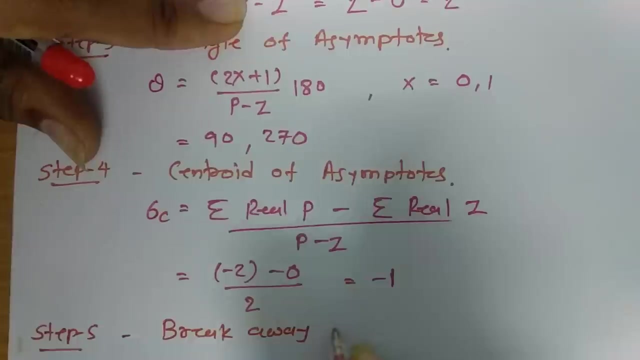 0, that is 2.. So this will be minus 1.. So centroid of asymptote, that is minus 1.. Now next step is to have a calculation of breakaway point. So next step, that is breakaway point Now. 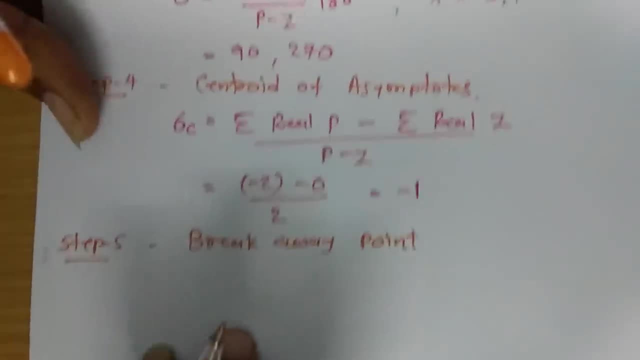 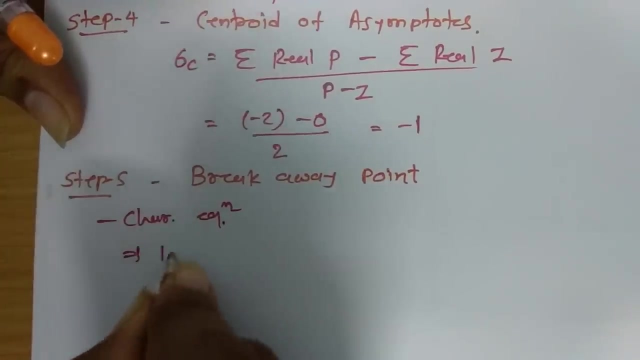 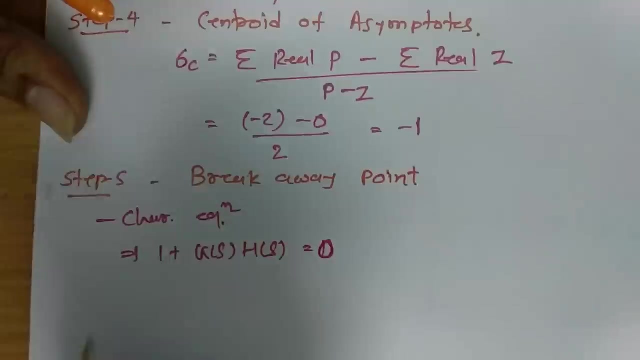 for breakaway point, we need to obtain characteristic equation. So characteristic equation, so that is 1 plus gs, hs is equals to 0. Now 1 plus gs is, in this case it is k divided by s into s plus 2, and hs is 1.. So, based on this you 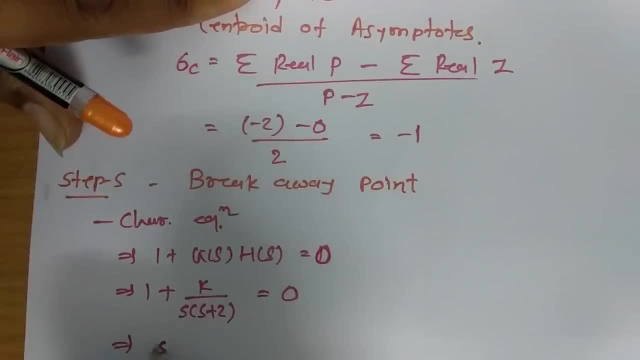 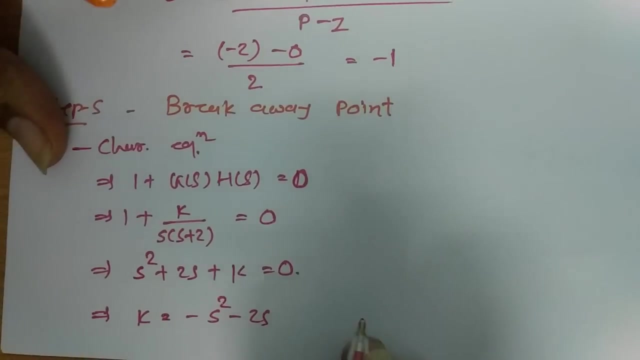 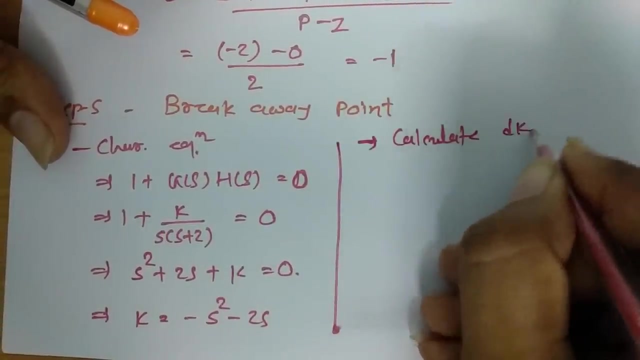 can say: characteristic equation is s square. So this is 1 plus 2s plus k is equals to 0. So now we will be calculating: k is equals to minus s square, minus 2s. Now next step is calculate dk by ds is equals to 0. So 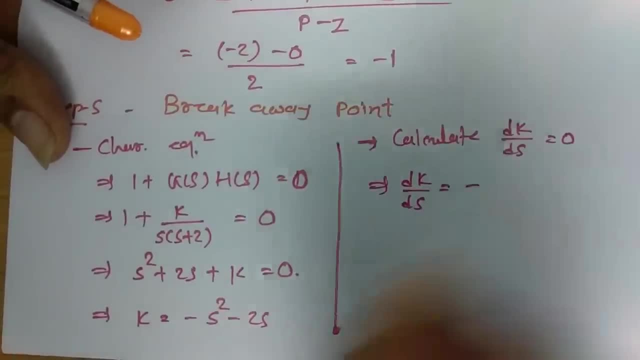 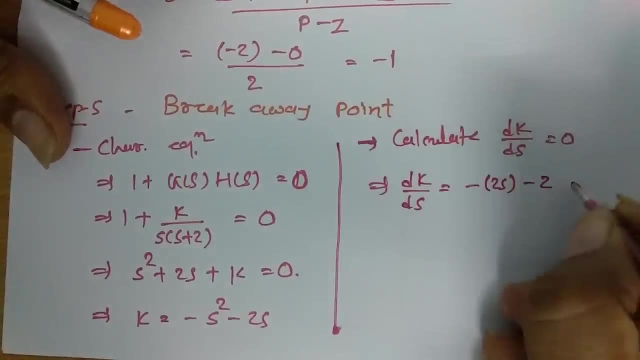 dk by ds over here, that is minus into s square's differentiation is 0.. So dk by ds over here, that is minus into s square's differentiation is 0.. So dk by ds over here, that is minus into s square's differentiation is 2s minus 2 into s differentiation is 1.. And if it is, 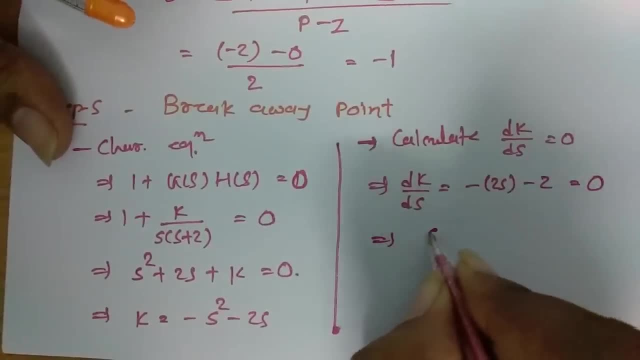 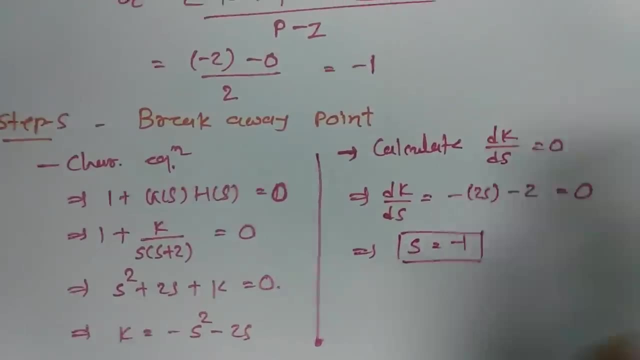 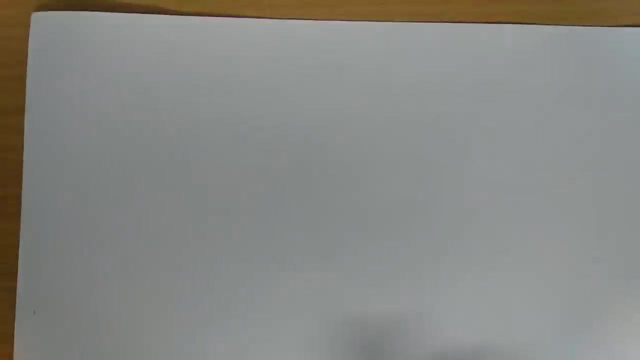 equals to 0, we can say s is equals to minus 1.. So we have breakaway point, that is, at s is equals to minus 1.. Now next step in this example is to have a calculation of intersection to imaginary axis. 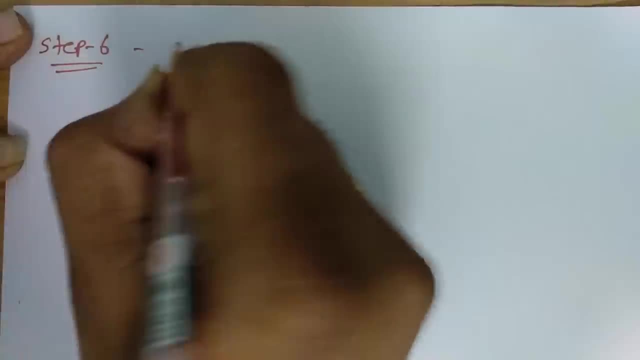 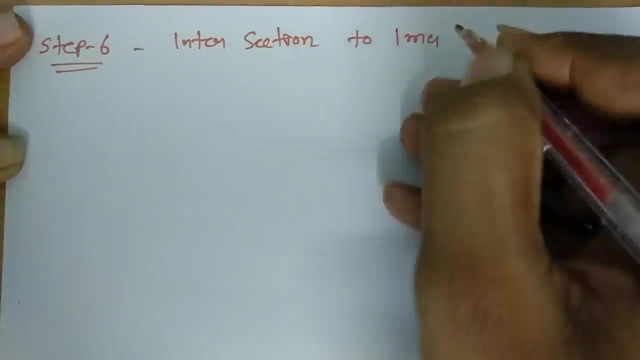 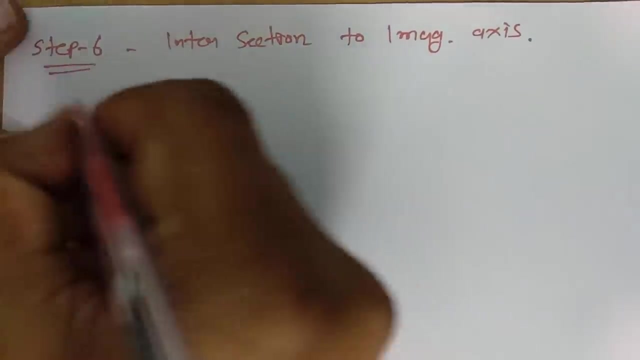 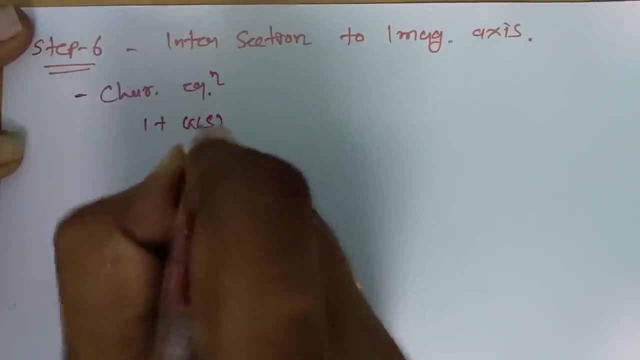 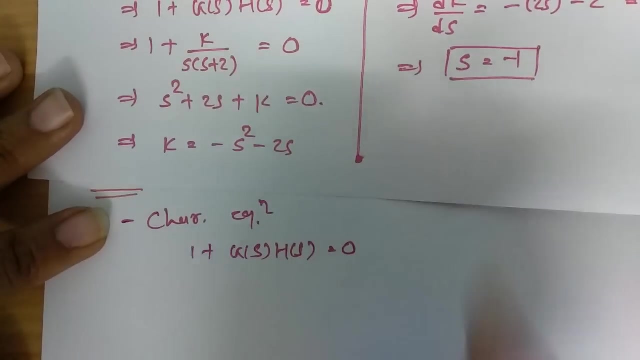 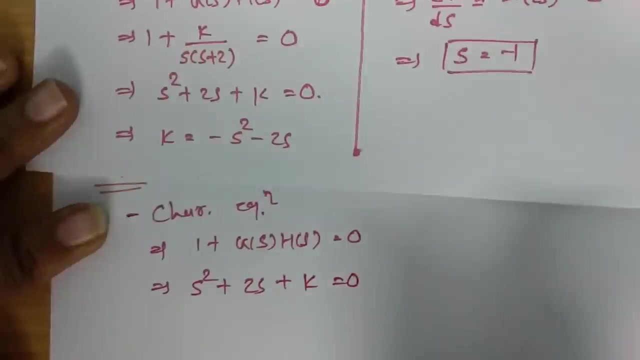 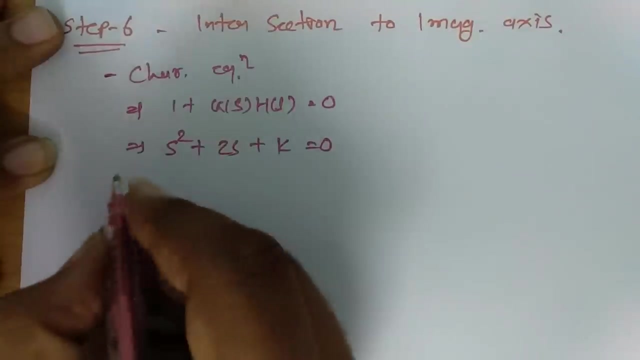 So step 6, that is, intersection to imaginary axis. So here, first we need to write down characteristic equation, and that is: one plus gs, hs is equals to 0.. In last session we We have derived this, So let us directly write it. So s square plus 2s plus k is equals to 0.. Now second step is to construct Routh array. 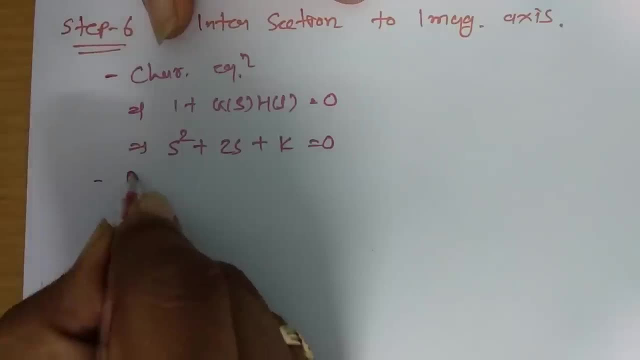 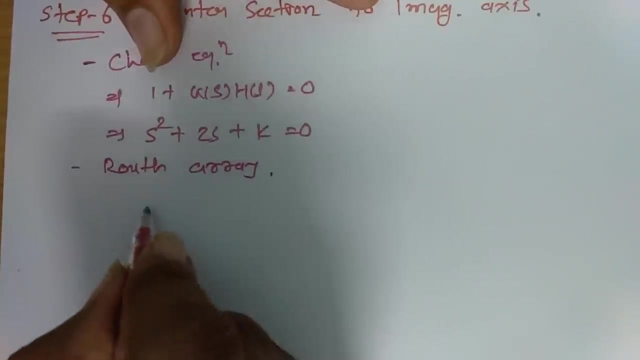 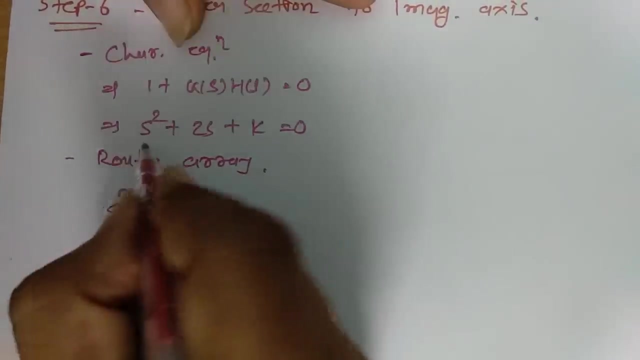 So Routh array based on this equation. So that is s square: s to the power 1, s to the power 0, s to the power 2, that is having 1 coefficient, skip 1, and that is having k and s to the power having 2 coefficient and skip. there is nothing. 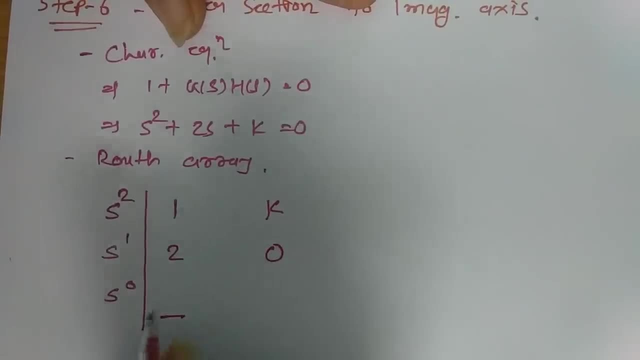 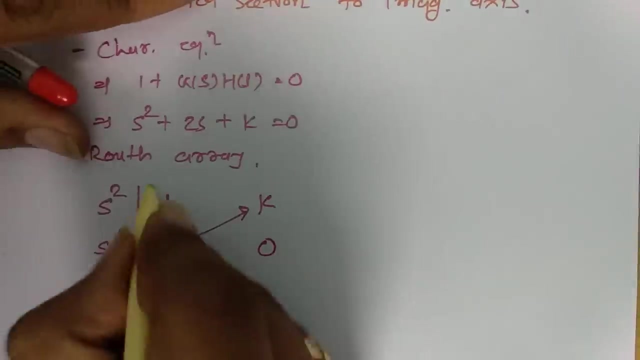 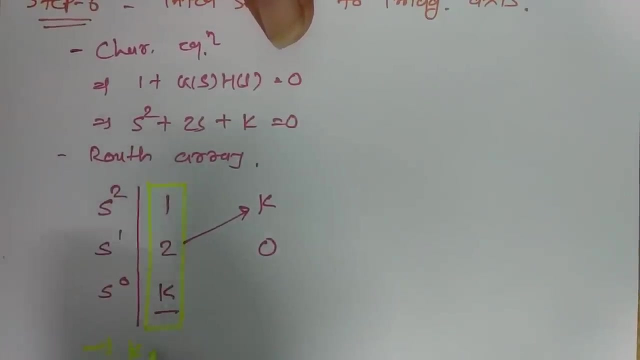 So over here it will be 0.. So next coefficient, that is this, which will be 2 into k, minus 1 into 0, divided by 2. So that will be k. So here for a stability, we have value of k that should be greater than 0 and there is no intersection to imaginary point. 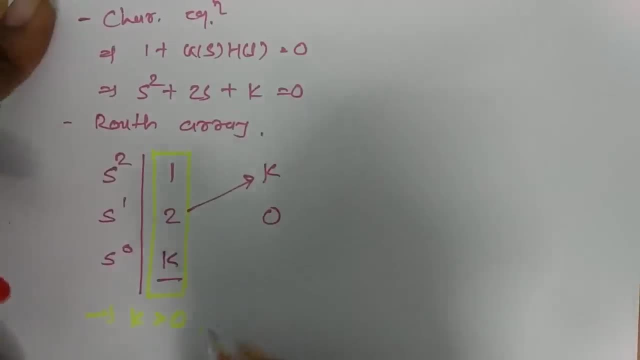 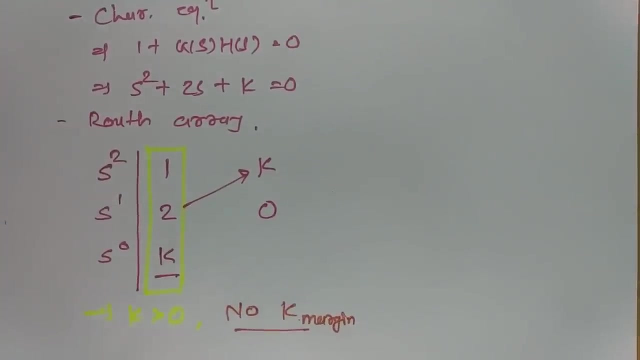 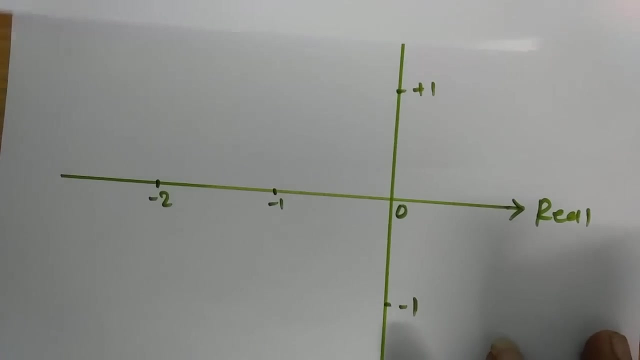 The reason is there is. So there is no marginal cable, No k marginally stable system, So we do not have any intersection to imaginary axis. Now, after having all those steps, let us have a plotting of root locus. So let us have a plot of root locus. 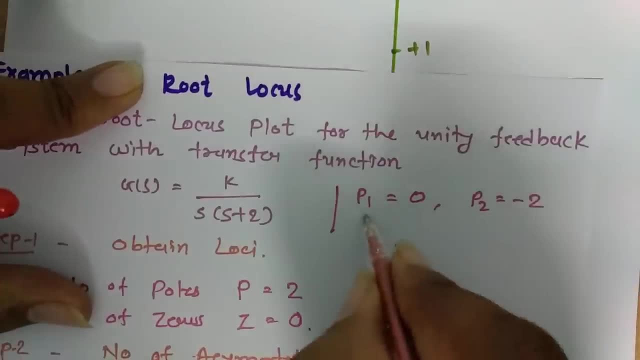 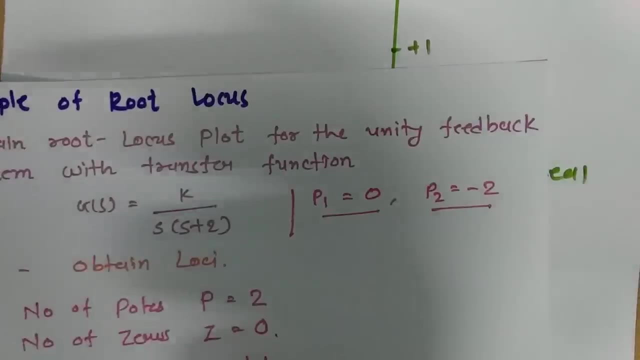 So in this system we were been having 2 poles. So in this system we were been having 2 poles. So let us place those 2 poles. 1 pole at s is equal to 0 and 1 pole at s is equal to minus 2.. 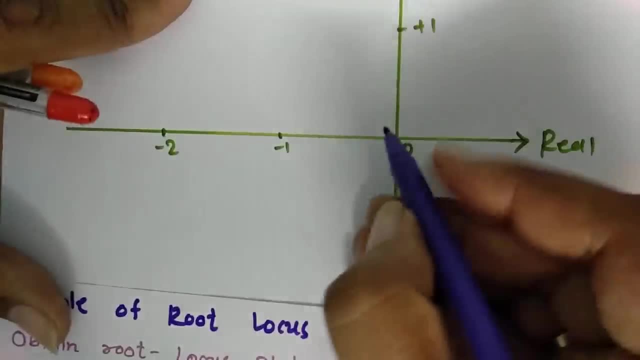 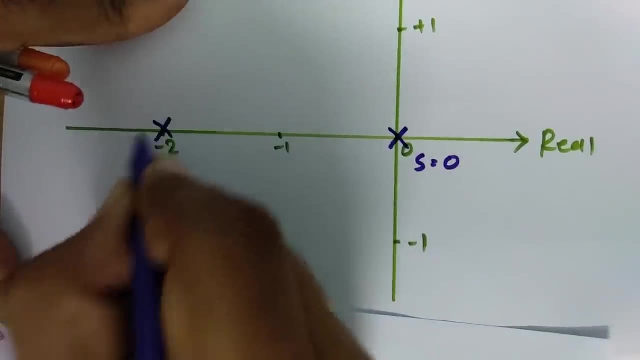 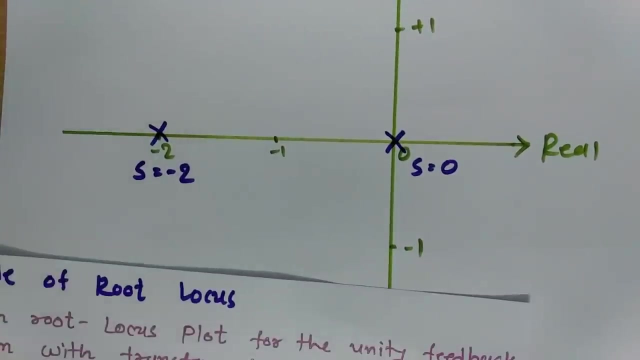 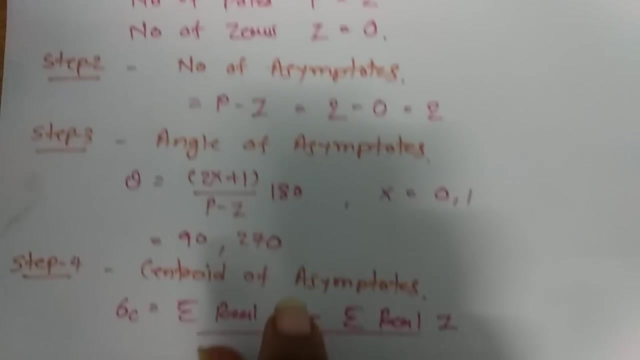 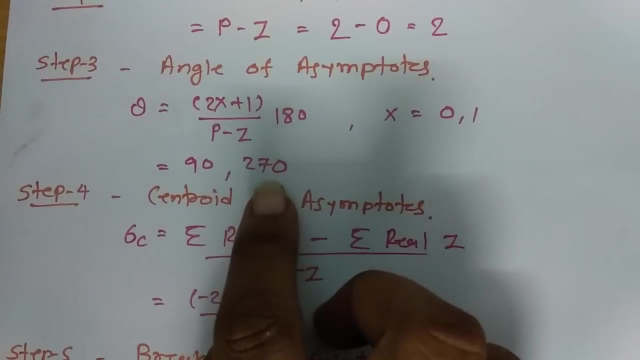 1 pole at s is equal to minus 2.. So here we have 2 poles. one is at s, is equal to 0, and here another pole is here, that is at s is equal to minus 2.. And there is no zero. And in this example we are having two asymptotes. One asymptote is having angle 90 and second asymptote is having angle 270. And centroid of asymptote that is at minus 1.. 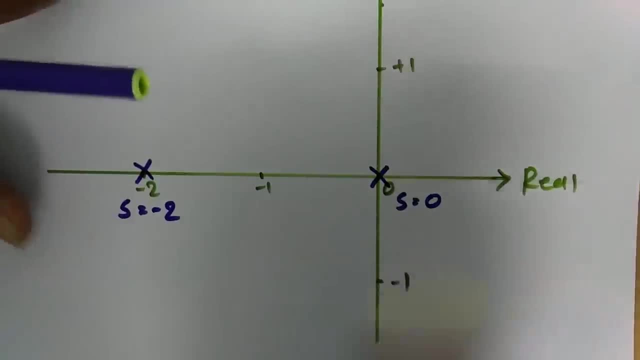 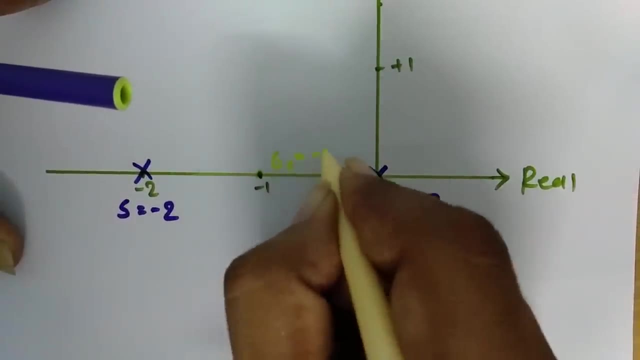 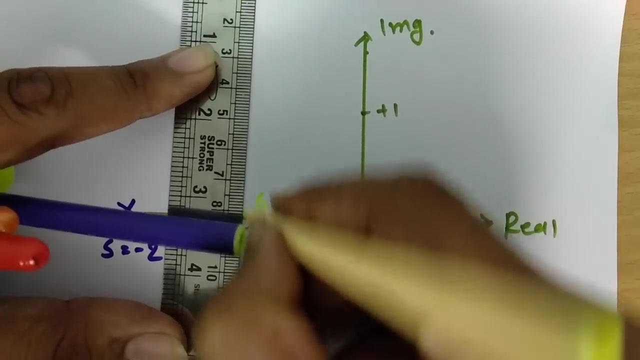 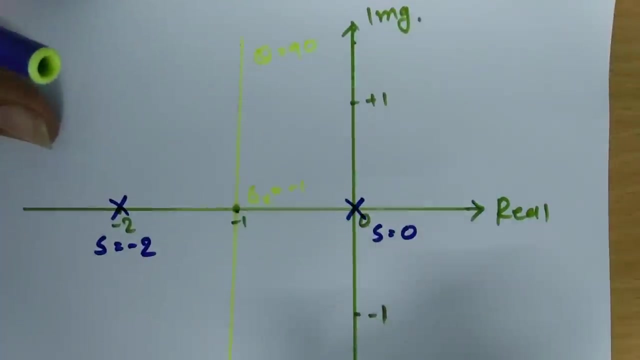 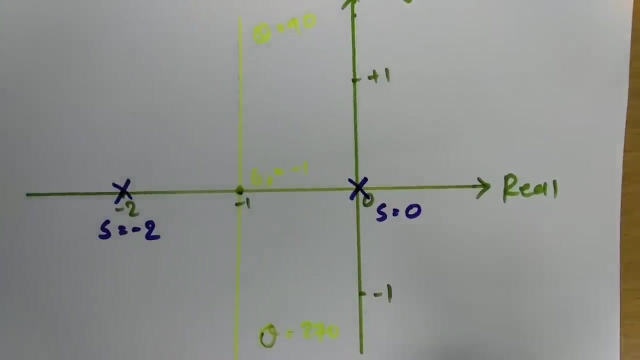 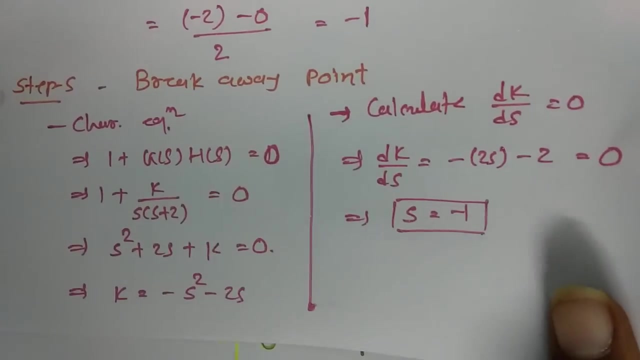 So over here we have centroid of asymptote, So centroid of asymptote, sigma c, that was there at minus 1.. And angle of asymptote that was there at theta is equals to 90 and at theta is equals to 270.. So this is what we have computed. And then we have seen breakaway point. So breakaway point that was there at minus 1.. 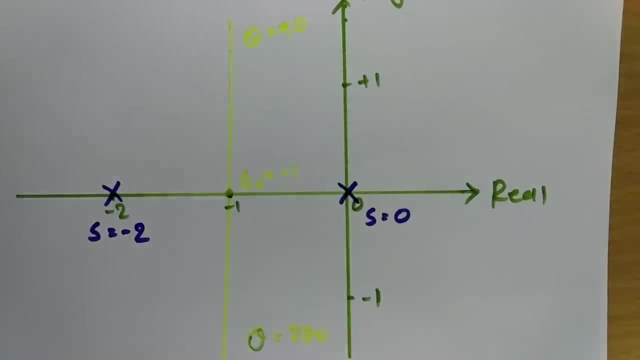 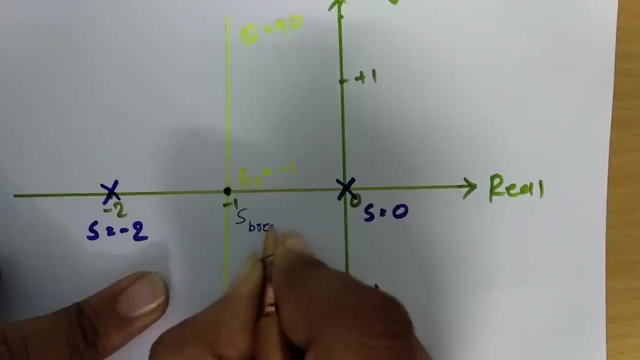 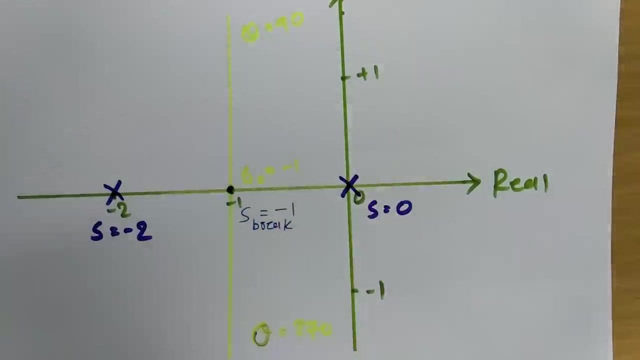 So even I will have to say S break. I am writing it, for breakaway point that is at: S is equals to minus 1.. So suppose S is equal to minus 1.. So centroid is at minus 1.. Breakaway point is at minus 1.. 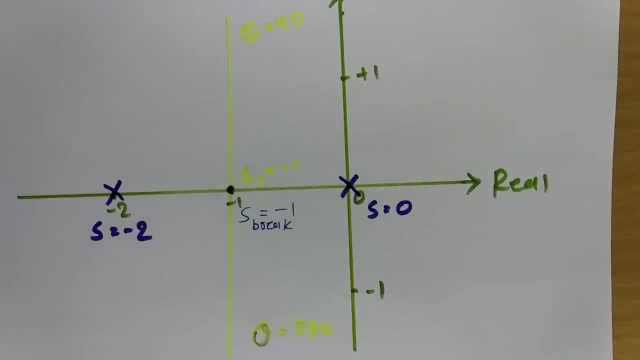 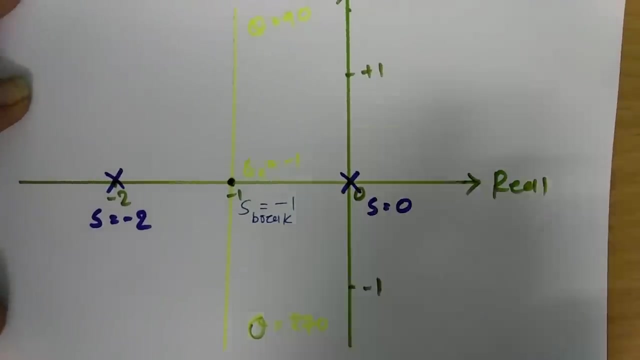 And angle of asymptotes are there at 90 degree and 270 degree, which we can see it over here. Now how to begin with example for plotting of this after calculating all those datas. So remember always line of root locus, that will always emerges. 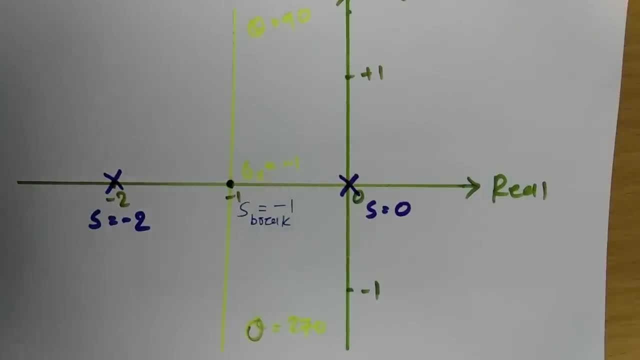 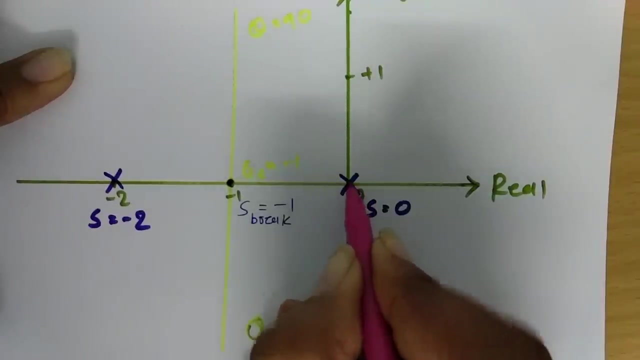 From poles and that will try to enclose to zeros And if number of zeros are less, in that case that will go to infinite. So line that will begin from both of this poles And that will go to breakaway point. And one more thing that we need to remember: from one pole, one line will emerge. 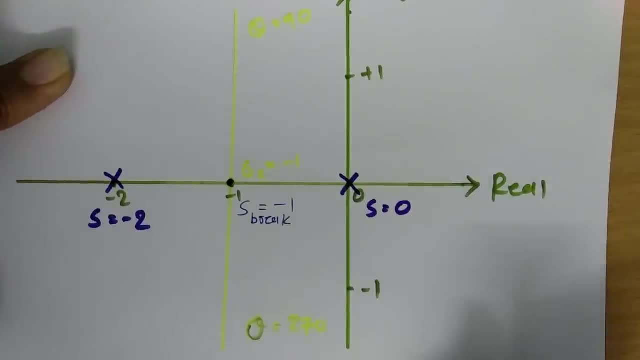 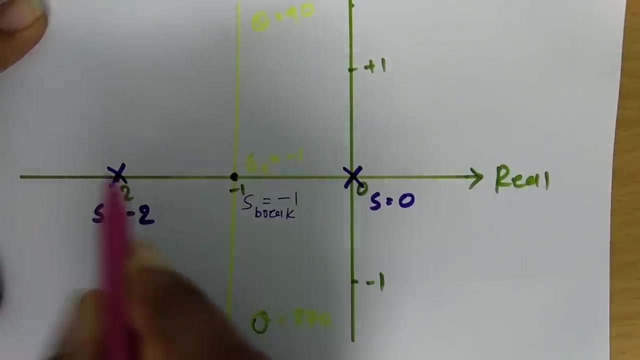 So from one pole two line cannot emerge. From one pole only one line can emerge. So from here only one line will emerge. And basic first rule of root locus is root locus. plot should be always symmetric with respect to real axis. So definitely from here, whatever line is getting emerged that will go in this direction. 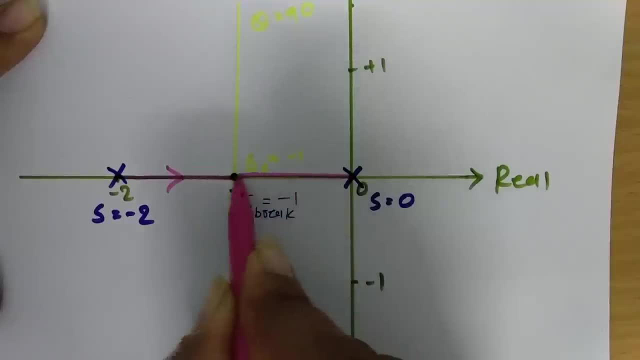 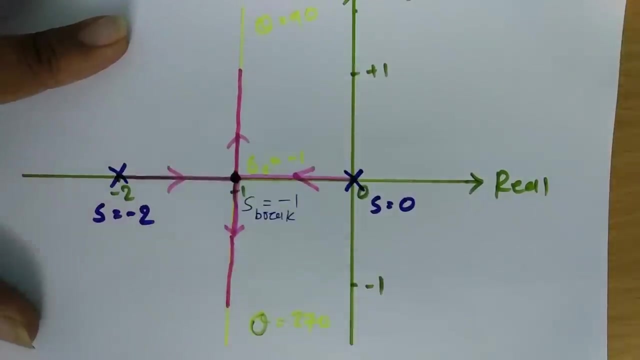 And the line which is emerging from this, That will go in this direction And that will get breakaway at this point And after getting breakaway now, it will be moving towards asymptotes. So see, that is how it is moving towards asymptote. 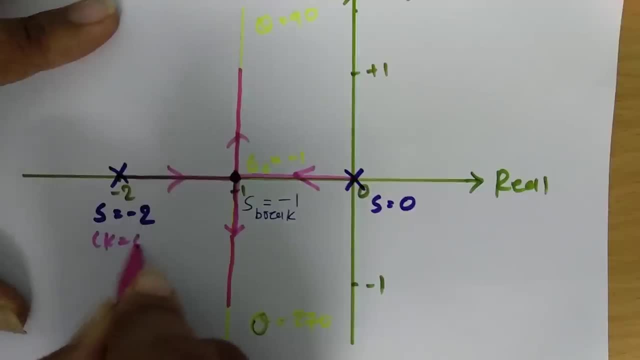 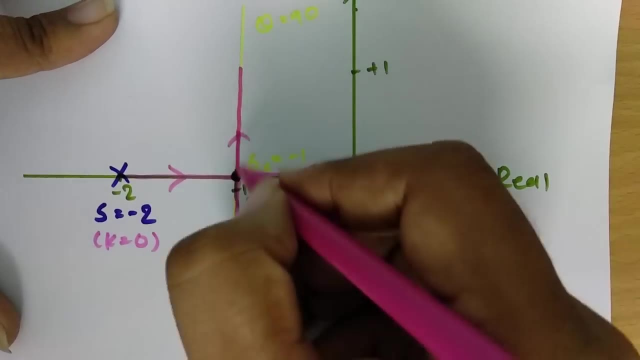 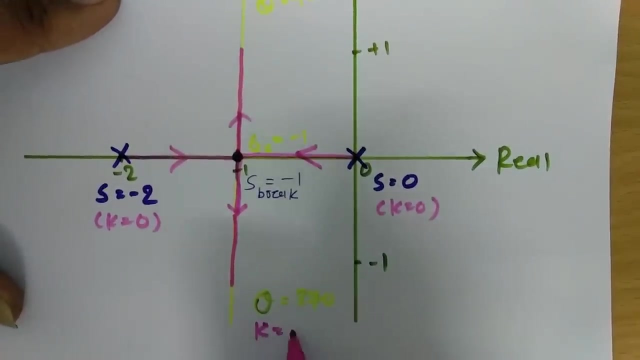 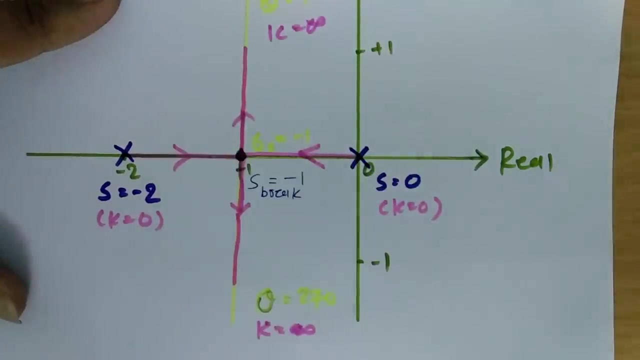 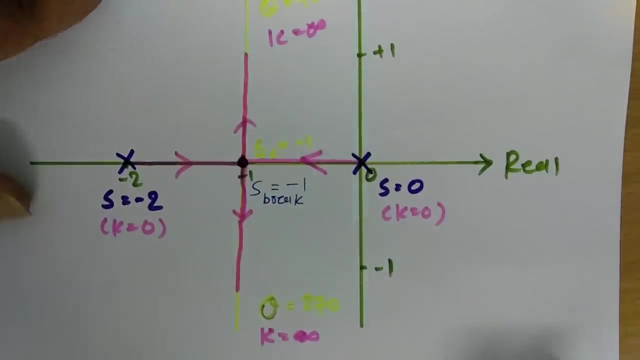 So ultimately, over here at pole, k is equals to zero And as it moves towards infinite, there will be k is equals to infinite. There will be k is equals to infinite. So that is how it is getting moved. So this is what the consideration which we need to see when we solve root locus example.